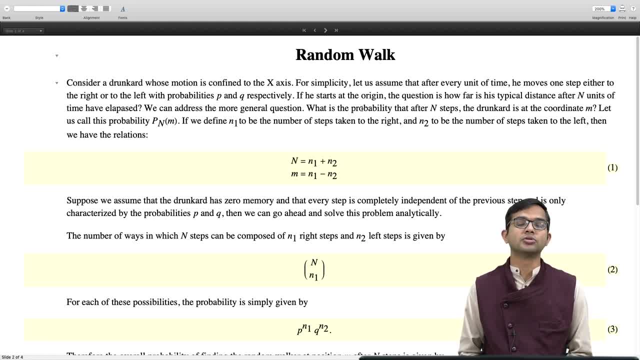 say he is confined to live on the x-axis, right? I mean, of course you can live on the x-axis. you can generalize this to higher dimensions. Suppose he is confined to walk along the x-axis, but at every unit of time, so he doesn't keep on moving. it is not continuous. 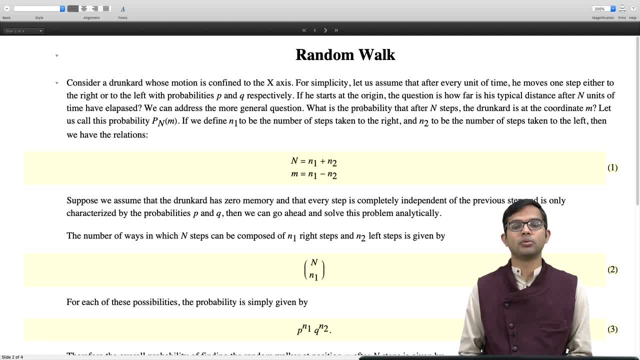 motion in time or space. we will consider the discrete problem first. So he can be either at the origin or he can be at plus 1,, plus 2,, plus 3, so on. right, in some units doesn't matter what. And time also moves forward in units of. you know one unit which could. 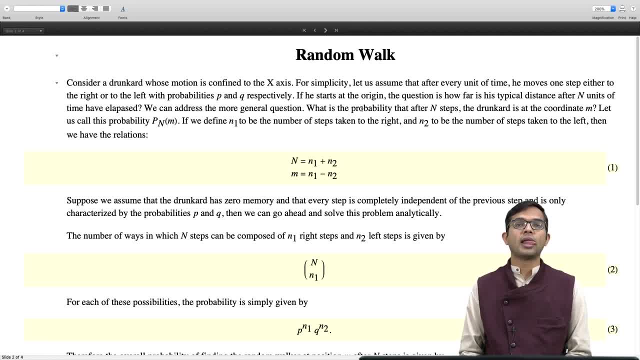 be whatever- one second or a minute or so, Or whatever you want to choose- And after every unit time. so our friend makes a choice whether to go to go right or go left. And so let's say, after capital, N, number of steps. 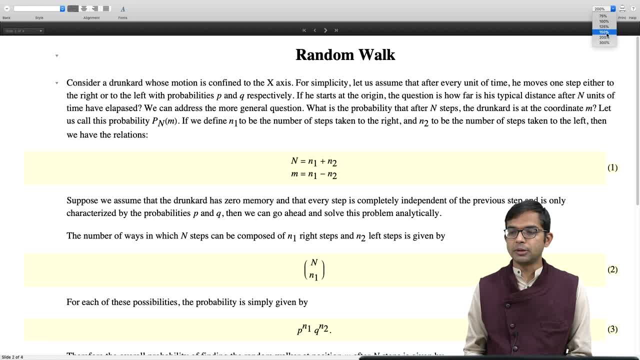 so we want to ask how far it has? what is the typical distance which our friend would manage to cover if he is given, you know, N steps right? So this is the type of question. It is a. it is a stochastic, random variable. it is not going to be, it is not going to. 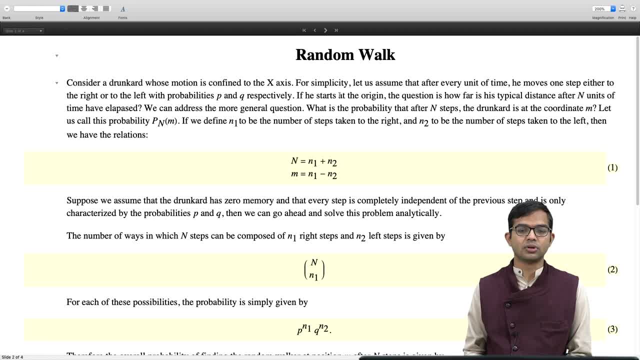 be. there is no definite answer for exactly where he is located is not something that you can calculate, because there is a. even he doesn't know where he will be exactly precisely after N steps, But it turns out that you still know a surprising amount of information. you. 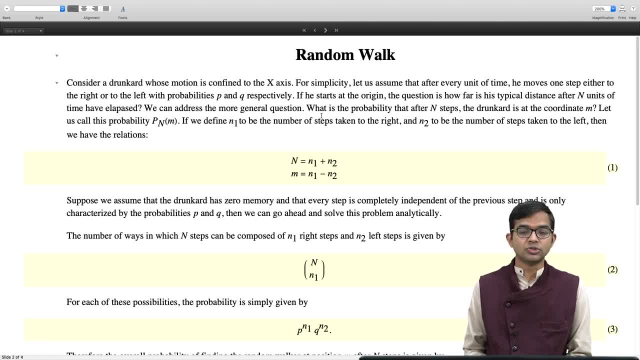 know in terms of you know the average location or average distance from the origin, and so on. You can ask a lot of questions and there are very precise answers to you know the some of these questions one can formulate in a stochastic way. 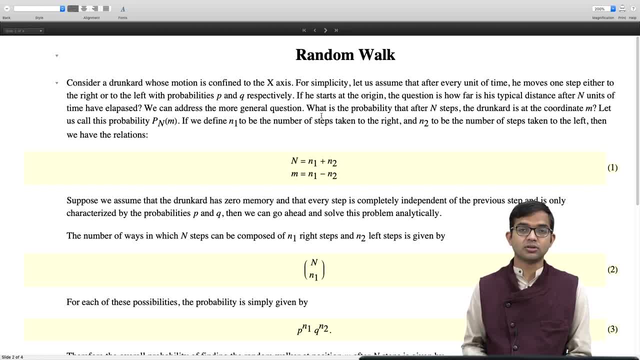 So that is the beauty of you know stochastic methods already comes out in something very simple like the random walk problem. So let us say that N1 steps are taken to the right and N2 steps are taken to the left right. So clearly, capital N must be equal to small. 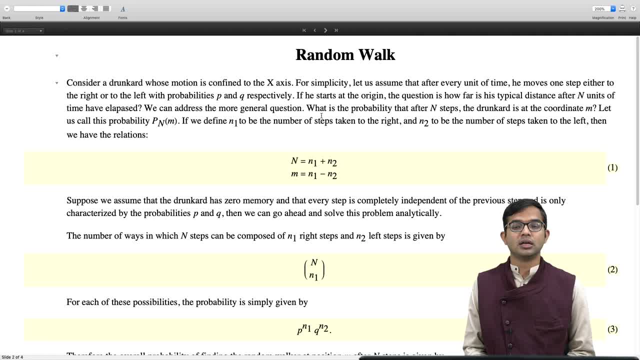 N1 plus small N2.. Because if N1 is, there is no option of not taking N1, right. So N2, there is no option of not taking a step right. That is the simplest model we are considering. You can also make this model a little more complicated and say that you know with some 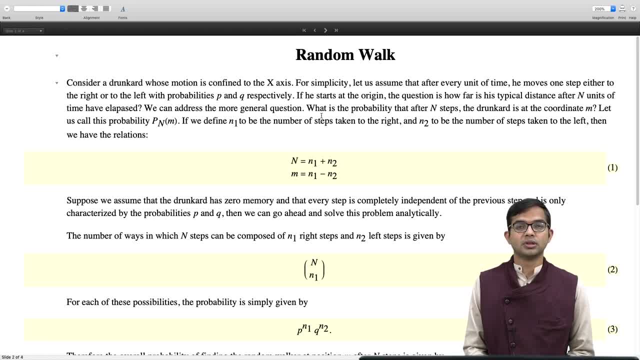 probability. you know some other probability which you know is such that P plus Q plus this new probability that we are introducing, is equal to 1.. The person stays at a location, right, You can say that with probability P he moves to the right and with probability Q. he moves to the left And probability N1, N2, N3, N4, N5, N6, N7, N8, N9, N11, N12,, N12, N13,, N13, N14,, N14, N15,, N15, N16,. 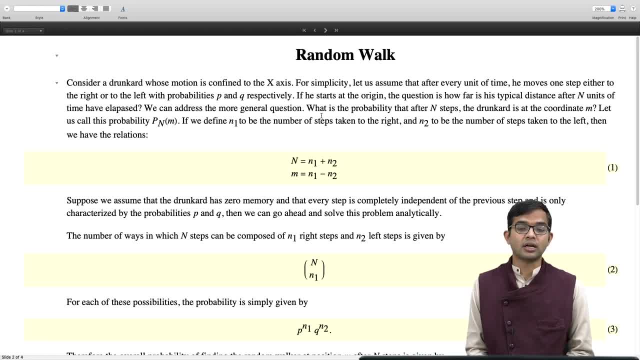 N17, N18, N19, N20.. So that we are considering- We are not considering it as P plus Q plus Q tilda. let us say He stays where he is, So that P plus Q plus Q tilda is equal to. 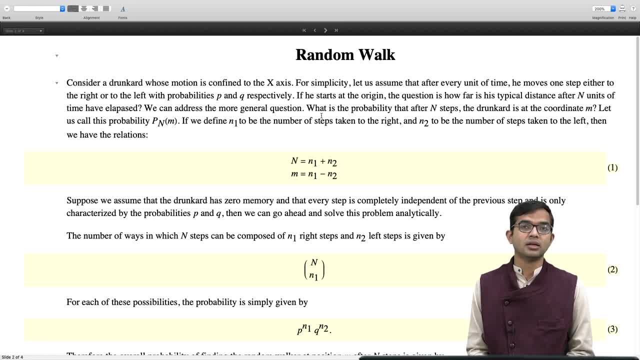 1.. So that option we are not considering. here We are saying that P plus Q equal to 1, and so the person either moves to the right or to the left at any every time, instant when a decision needs to be made. So therefore, capital N is equal to N1 plus N2.. So a quantity 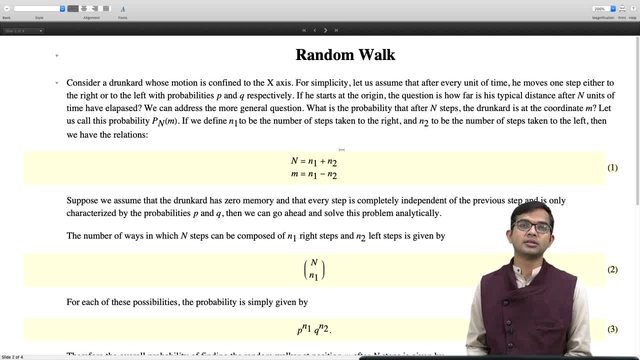 of interest for us is small n, which is just simply defined as N1 minus N2.. So you are. you know what is the typical distance that our friend manages to cover. as a function of time, right, It could be a negative number, but you will see in some time that actually. 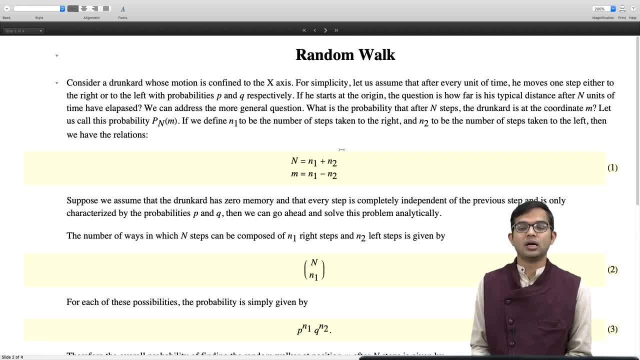 we care about the modulus of m or, even more convenient, is actually m squared. So you are interested in finding out what is the typical distance squared of. you know, distance covered by this person as a function of capital N. If you move, if you take capital N, m number. 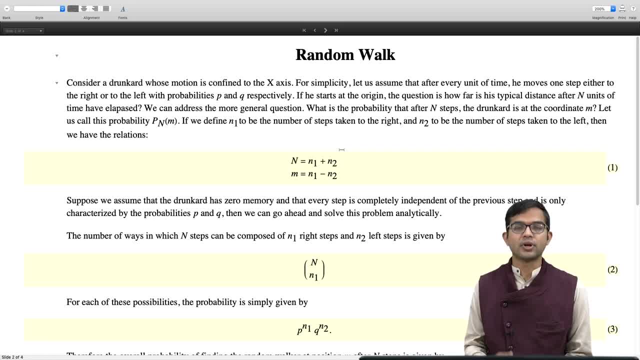 of steps. what is the typical? m? right, It is a. in fact, it will turn out that you can compute the full distribution itself, the probability distribution. Okay, so let us say that there is no, no memory right in the motion of the random walker. 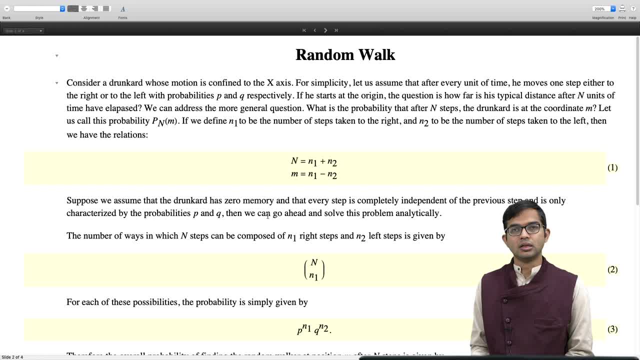 So at every instant of time, the person basically does not care about what they did in the previous step. right, So they make. you can think of it as as tossing, Tossing a coin every time He goes to a step and then, before he makes up his mind next. 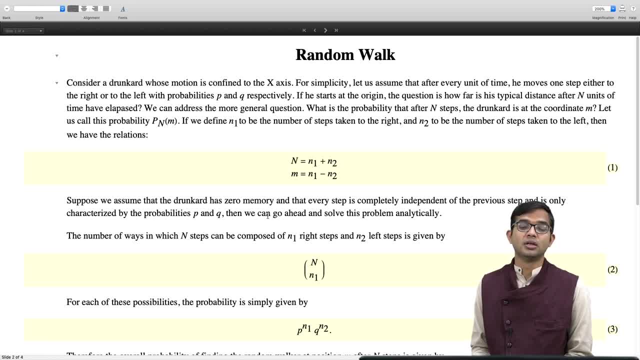 time he just tosses a coin and with probability p, the toss is going to give him heads, and which he will go to the right, and with probability q, he is going to get a tail and he is going to go to the left right. So so these kinds of you know this type of a model can well. 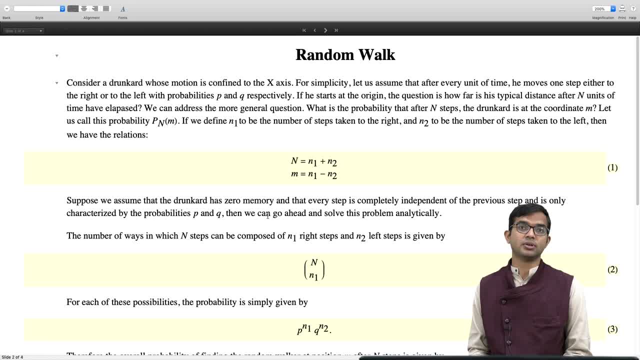 be applied to the motion of stock prices, for example. right, But there it turns out that this kind of, this kind of memory less model perhaps, is not the most accurate, although some people have argued. So. there are, you know, mathematical models of the of stock prices, where people 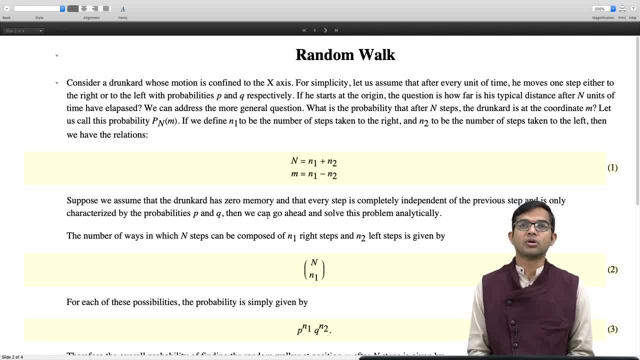 argue that it is basically a completely random walk. right, And you know, there are anecdotes where you know there was a group of academicians who just took up, cooked up data using random walk and then through random walks, and then they just, you know, showed this data and 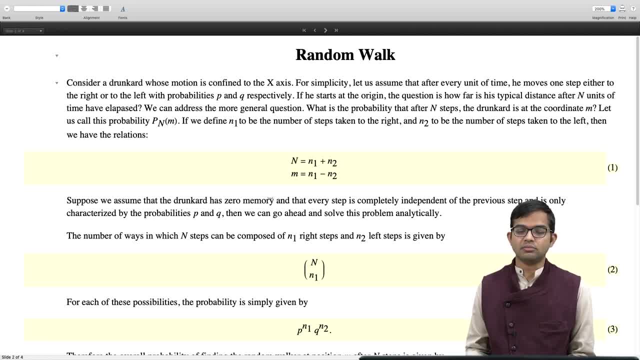 put this data to some financial analyst and they they predicted: oh this, we see a pattern here and then you should put your money in here and it is going to go up or whatever, right. So and basically their argument was that their data generated from random walks. 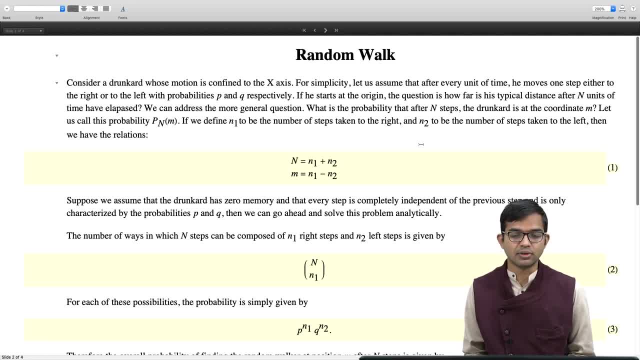 were basically completely indistinguishable from realistic data where people claim that you know there are, there is some hidden order there. right, which is predictable? right, Predictability is what is not possible, Right? So it is a very difficult thing to do So. 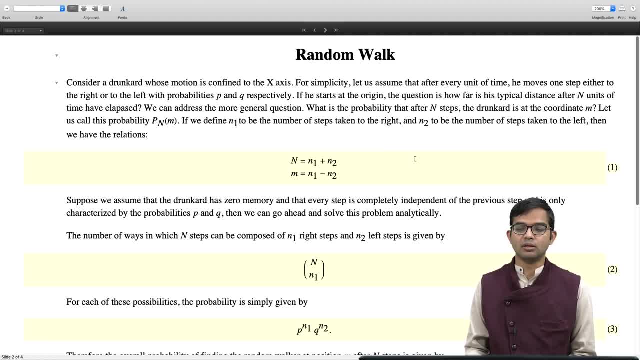 of great interest in the context of stock price. But it turns out that in fact there are other academic discussions where people have argued that in fact there is. it is not really a random walk. there is some predictability involved and in fact that has to do with the fact that there is often some memory in your, in the 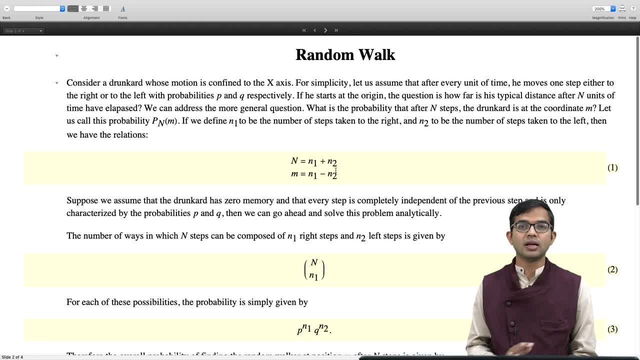 motion of stock price or whatever at every instant. it is not going to be completely cut off from what happened in the prior instance. So typically there is going to be some speed associated with it and it keeps going in a certain direction, and then, of course, there is a randomness associated with it as well. 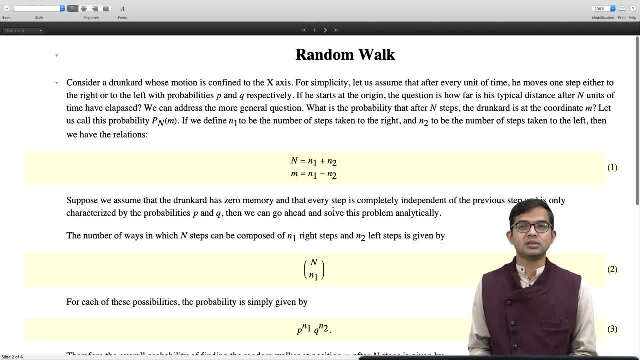 and there it. you know, if sufficient people start seeing a trend, then they try to exploit it and therefore the trend gets reversed there. So in some sense the whole system One enforces, a certain amount of randomness is an essential aspect of that system. But okay, so that is just a small digression into how a model of this kind can be applied. 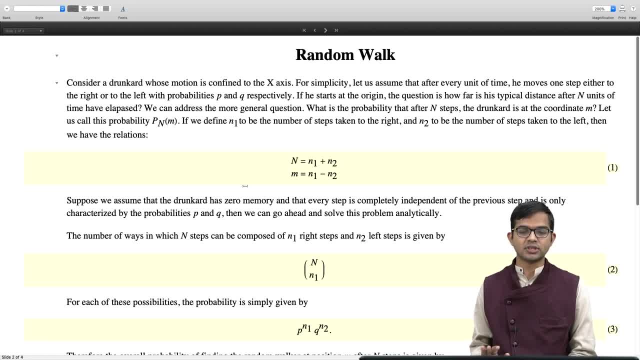 in the context of stock market. But for our model we are very, very simple, So we do not have any memory effects here. at every instant it is a fresh coin which is tossed. with probability P, you go to the right, and with probability Q you go to the. 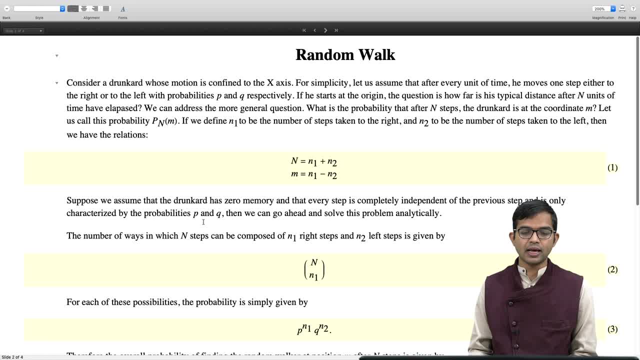 left. So the number of ways in which capital N steps can be composed of small n. 1, n, 2, n, 3, n, 4, n, 5, n, 6, n, 7, n, 8, n, 9, n, 10, n, 11, n, 12, and so on and so forth. 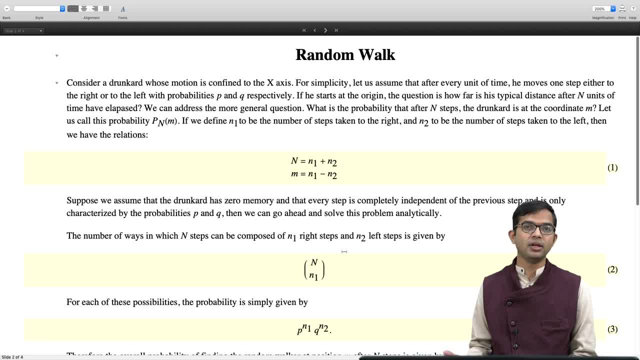 So it is very simple. So the only way to compose those small n 1 right steps and small n 2 left steps is simply n choose n 1 right Now. for each of these probabilities, the probability is given by you know, P times, P times, P times. 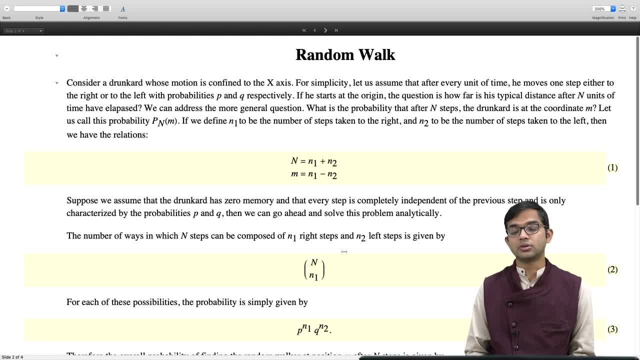 P, so on n 1 times and Q times, Q times, Q, so on, n 2 times. So you have to tag along all these various possibilities, you have to count them, which we already did n choose n 1 times. p 1 to the power, n. 1, n, 2, n, 3, n, 4, n, 5, n, 6, n, 7, n, 8, n 12 times. 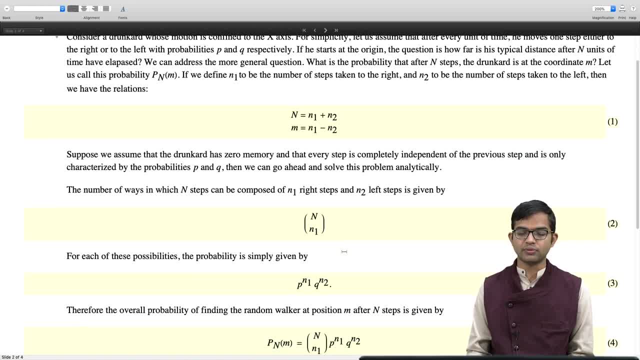 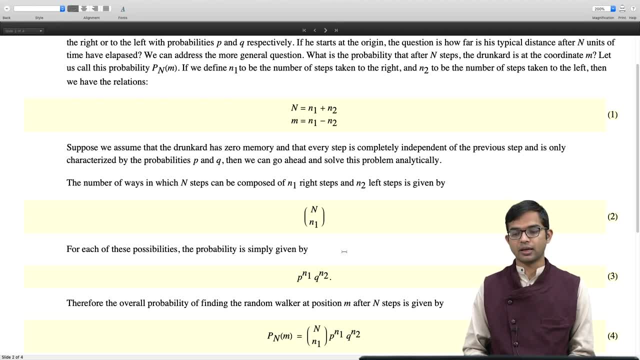 to the power, n1 times q to the n2.. So therefore, in fact, that is all there is to it. Therefore, the overall probability of finding the random walker at position m after n steps is simply given by n choose n1 times p to the n1 times q to the n2 right. So this is already a bit. 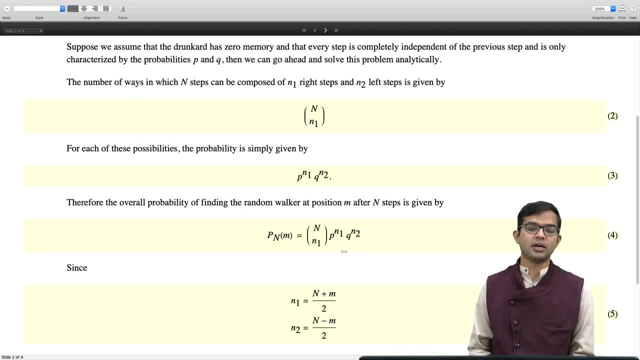 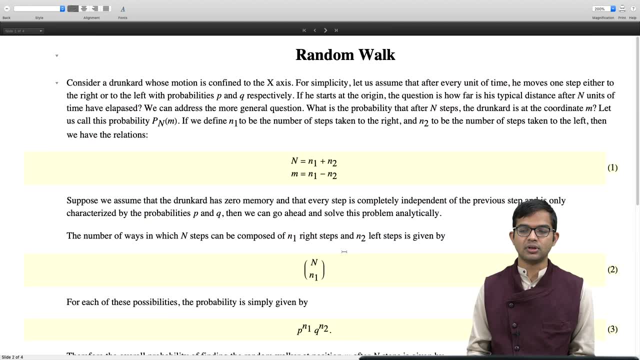 of a result. So now we can invert this n1 and n2 and write n1 as capital N plus m by 2 and n2 as capital N minus m by 2. all I have done is just to solve for n1 and n2 in equation. 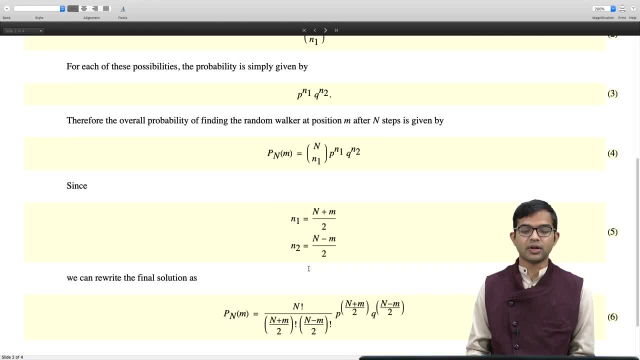 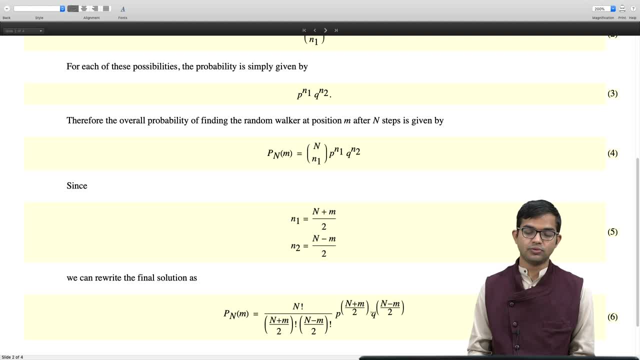 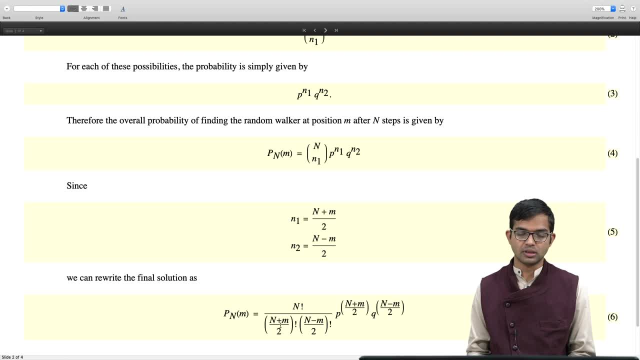 you cannot. you cannot have m odd right, So this is so, for example. so let us suppose just think of the case where you just walk once you take one step. if you take one step, then for sure you can. you could have gone either to the right or to the left, So there, 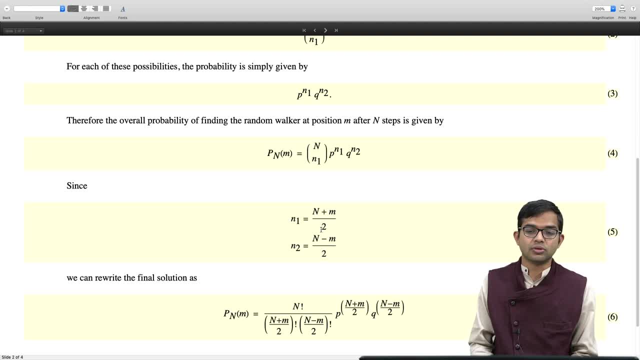 is no question of the walker being at 0, right? So the probability, so you can ask whether they are at 1 or whether they are at 3.. So after two steps, then for sure, you are guaranteed that your walker is going to be at an at an even position. there is no odd, there is no. 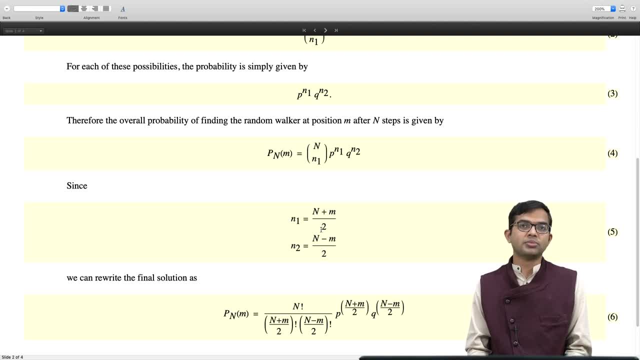 possibility of them being at the odd position. And the third step: they are guaranteed to be at either 1 or minus 1, or plus 3 or minus 3. all these possibilities arise, but for sure they cannot be at the origin. they cannot be at 2 or 4 or whatever right. So so this is. 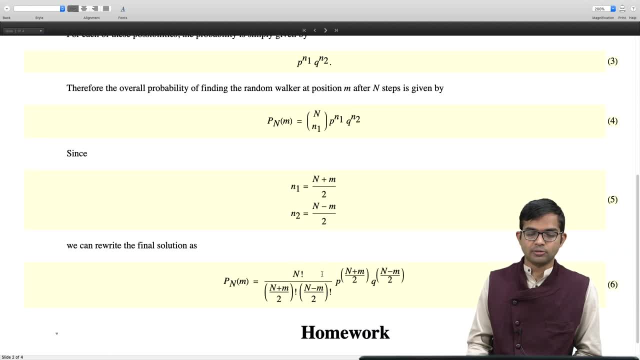 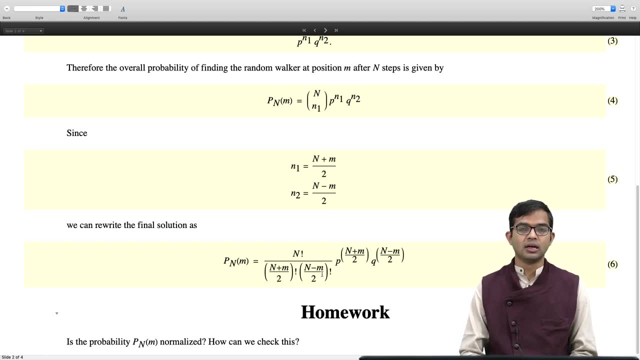 ingrained into this equation, right? So okay, so here is a homework question for you. how do you, how can you be sure that this is a reasonable probability here, right? So what, ah, Can you check this? is it already normalized or is there some more work one has to do to? 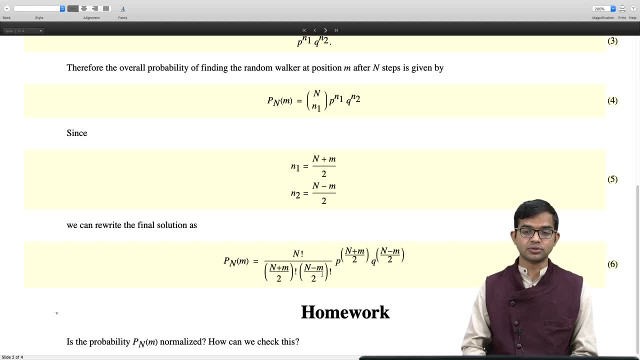 normalize it. So I am claiming that it is already normalized because I have used a nice argument involving probabilities to get to another probability, and I have. I believe that I have done my counting correctly, But you should check this and the way to check this is to just sum over all possibilities here, right? So probability is a quantity which 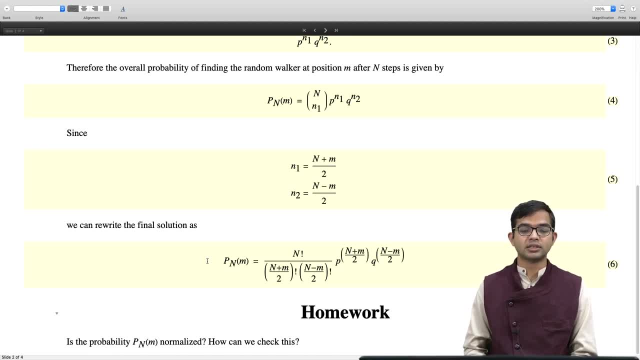 must add up to 1 if you ah, you know, sum over the entire sample space In this case. so m can only go from ah. The maximum value of small m is of course capital N right. So if all steps are taken to the right, then n1 minus n2 is exactly equal to m, because n2 is 0 right Now. on the other, 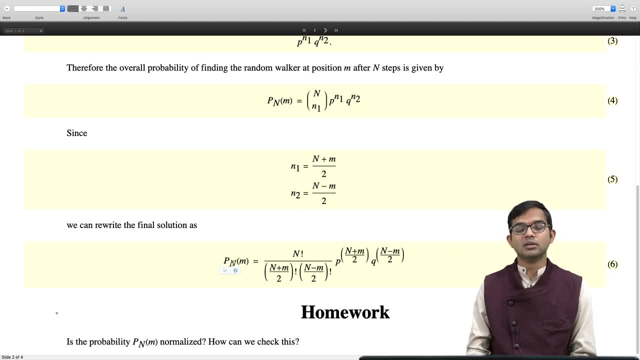 hand. if so, the the smallest value of n in magnitude is 0, but it can also be minus n. if all steps were taken to the left, it could be minus N. So this is one of the basic Buoyant. ok, Do you know why this is always possible? what? 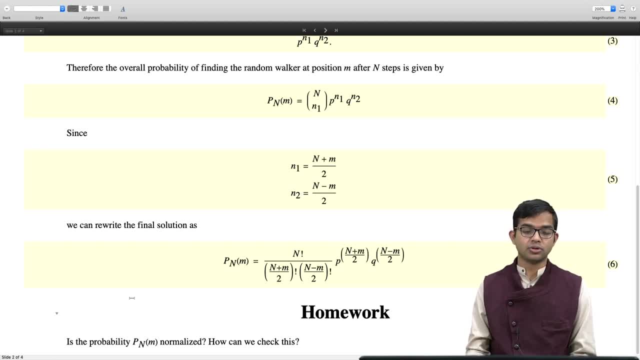 n over m. Why, Yeah, older, Sorry, not. So. therefore the jeden terms it has to be exactly 1 and n. So what you should do is just sum over all possibilities of m, first start small, take capital N to be 2 and 3 and 4 and so on, and then play with it for yourself and 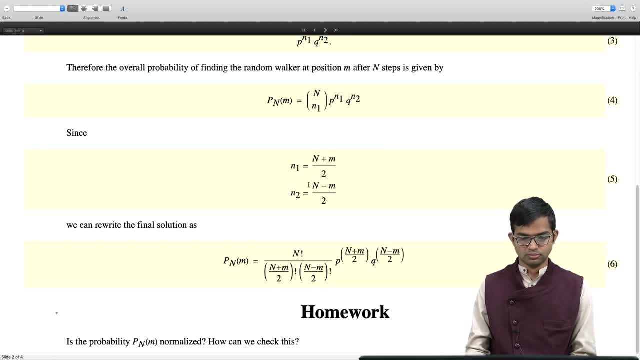 then you see a pattern why they should just sum up to 1, and then you will see that there is a simple, direct way to solve for this. that is homework for you. okay, let us move on. So what I want to do is show you some tricks here. some of you might have seen this, but 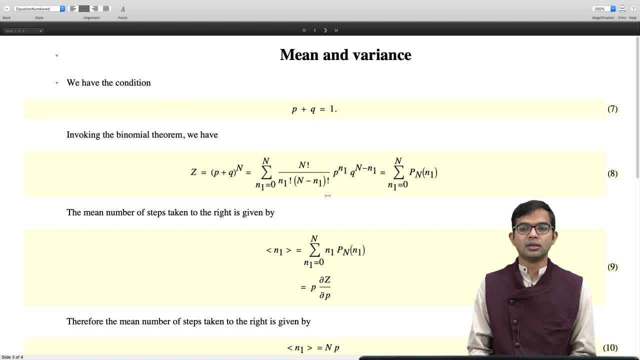 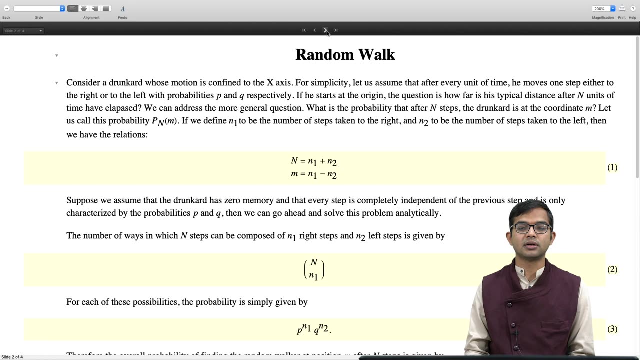 it is a very clever. you know the way to compute the mean and variance of this distribution. So we have the condition p plus q equal to 1, right, I have said it. but it was also sort of implicitly clear that there is no possibility of the random walker at any instant of time. 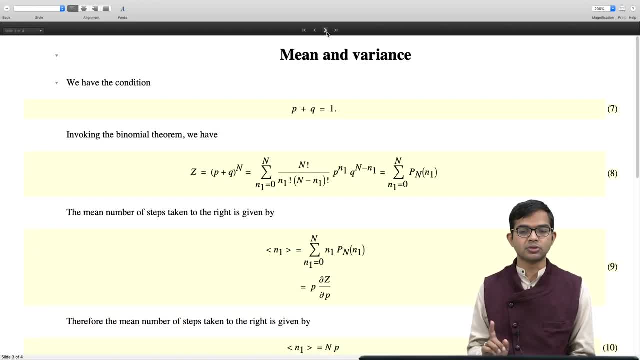 to not make a choice. he either goes to the right or to the left. therefore, p plus q is given to be 1,. right Now, consider this quantity, z, right? I mean, you will see in a moment why I am doing this. So I have: z is equal to p plus q, the whole power N. for now, you think of this as you. 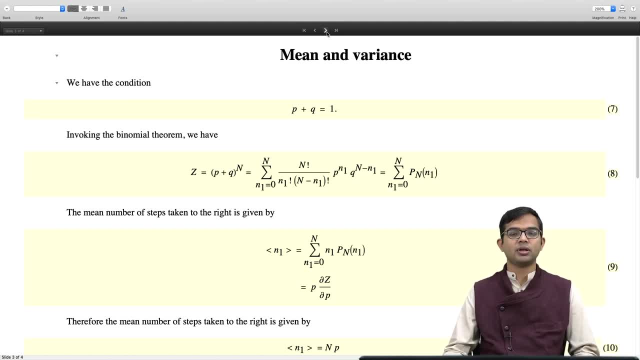 know just some two variables, p and q. you are not already putting p plus q equal to 1, we will do that later on. so it is just some trickery involved here, right? So I expand p plus q to the whole power N and write it as this series summation over N1, going from: 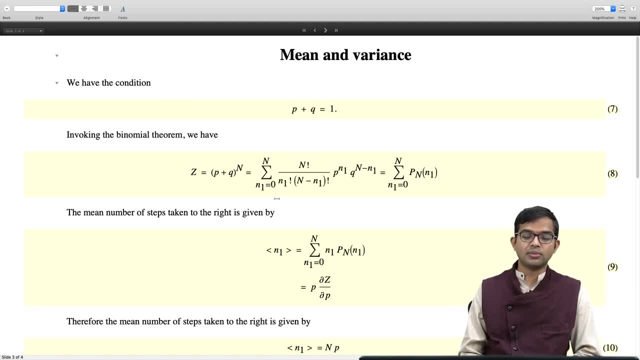 0 to N N. choose N1, which is N factorial, by N1 factorial times N minus N1, the whole factorial p to the N1 times q to the capital N minus N1.. So this, let me call this as equal to p. 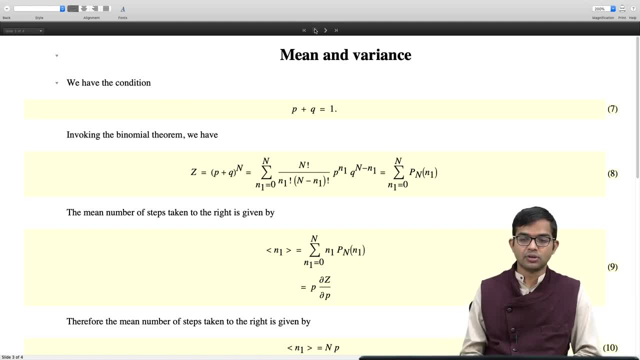 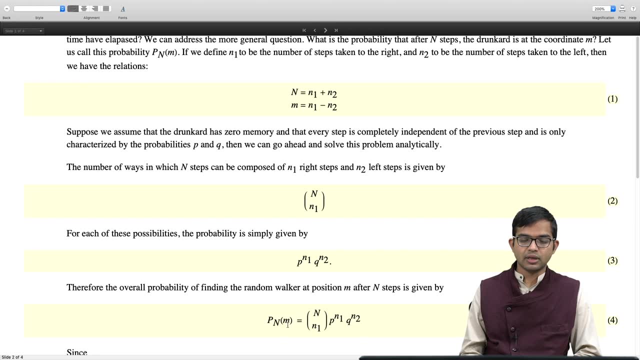 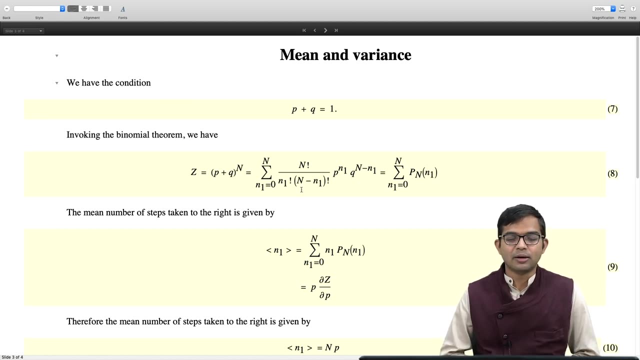 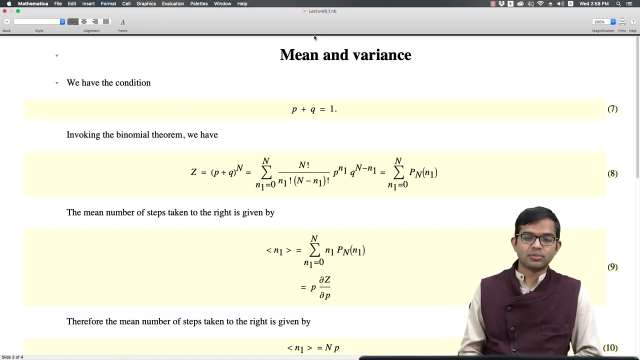 N of N1, because you see, this is exactly the expression I have for I have for my p: N of M or N1 is the same. So so, if you are paying attention, this already gives you a proof of why, Why this probability is normalized. you see that. so if you see that, do not see that. 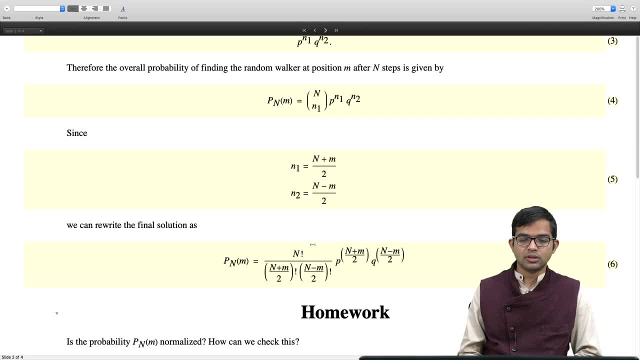 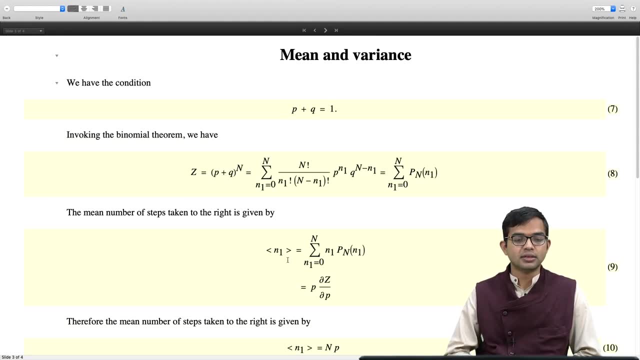 spend a minute. you can pause the video here and go back to this homework problem and then connect to this expression for z I have and then quickly check that indeed, it is a normalized probability distribution probability. okay, So the mean number of steps taken to the right. 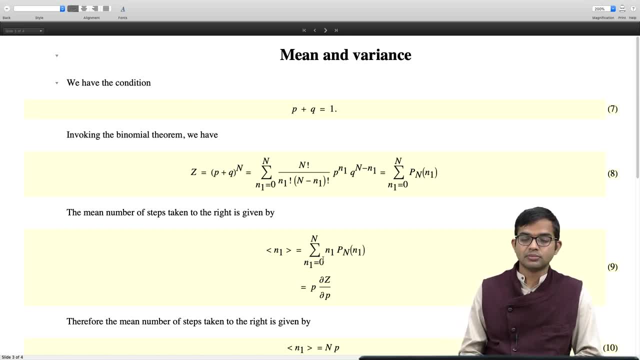 is just given by summation over N1 and it is you have to do N1 times pN of N1.. pN of N1, which you can see, that now you see the power of this expanding this type of a quantity called z. See, you think of this z as simply an algebraic expression For a moment. 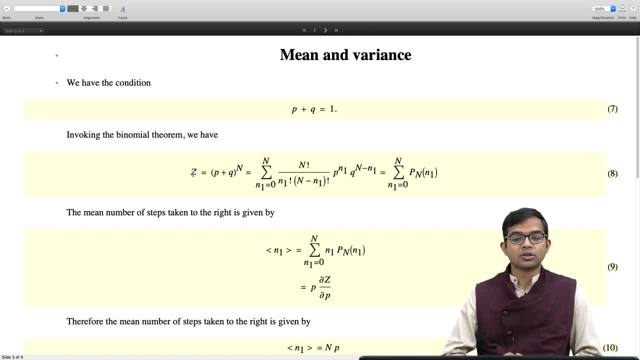 you are not supposed to, you are not supposed to put in p plus q equal to 1.. Do not think of it, as I am taking the derivative of 1 with respect to just think of it- as a derivative of some function of two variables: p and q. 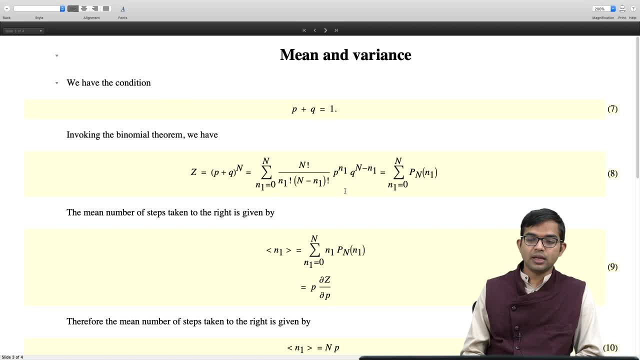 And then you just do Do z by doh p, then you see that you will get N1 times p to the N minus 1.. So you, this N1 here is, you know, it appears in the sum when you do this doh z by doh p, and then, but you, 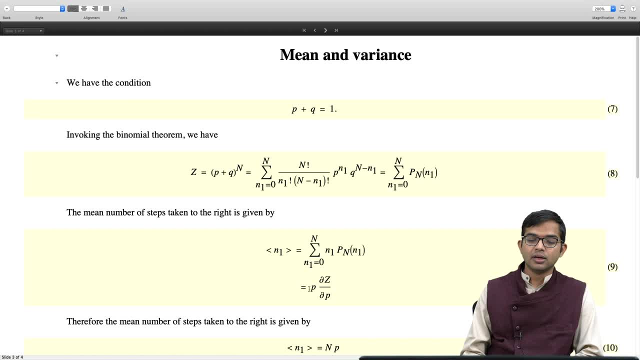 are losing a power of p. So you have to multiply by p so that you adjust appropriately for all the powers, and then you see, you can evaluate this expression. What I suggest is just doh z by doh p, and then multiply it by p and then check for yourself. 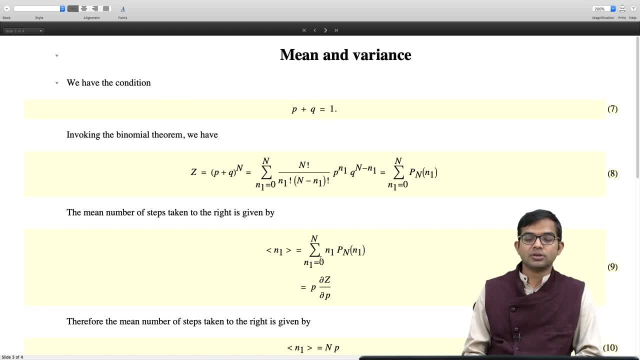 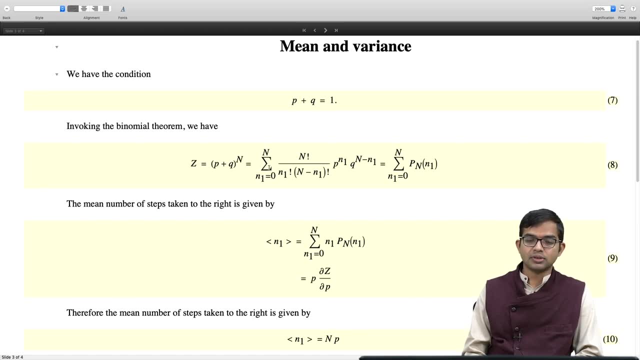 that, indeed, that is equal to this sum over N1, equal to 0 to N, N1 times pN of N1, and then you can, of course, very quickly evaluate it. now, Now that you have this, you can evaluate it, and then you see that the number of the mean 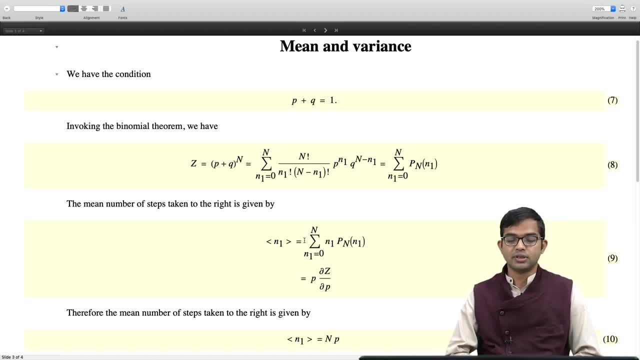 number of steps taken to the right is simply given by average of N1 is equal to capital N times p. Right, Ok, Because doh z by doh p is going to be just N. Yeah, you see that. so it is just you can. 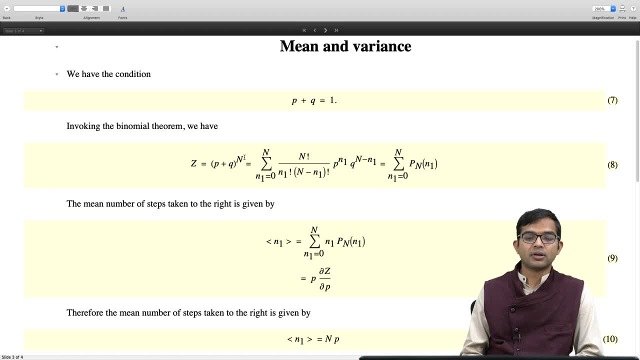 if you take a derivative, it is N times p plus q, the whole power, N minus 1 and p plus q. now you put in p plus q, equal to 1.. So it is. you will just remain with N for doh z by doh p. 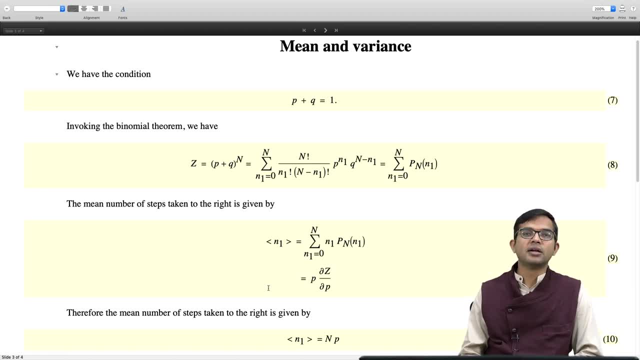 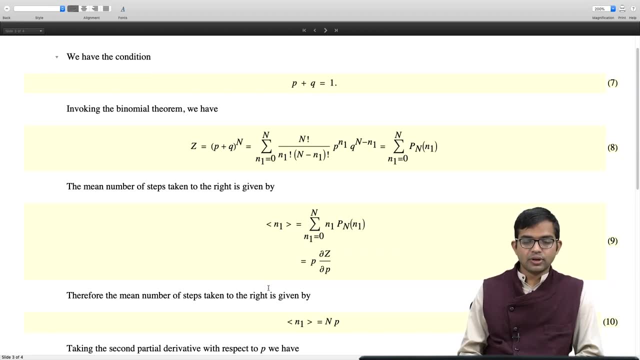 then it is just N times p. It is some clever trickery. there are surely there are other ways of doing this as well, But this is one nice way of doing it. Okay, You can go ahead and actually find the second moment as well. It is of great importance. 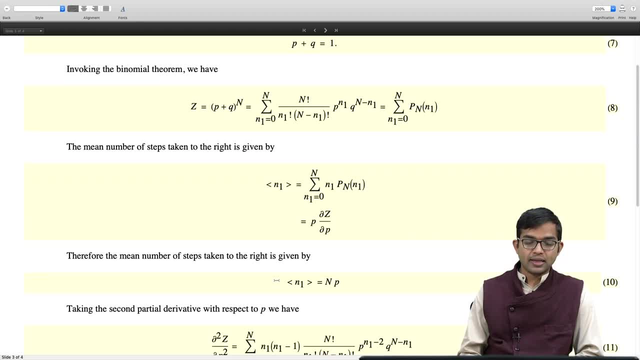 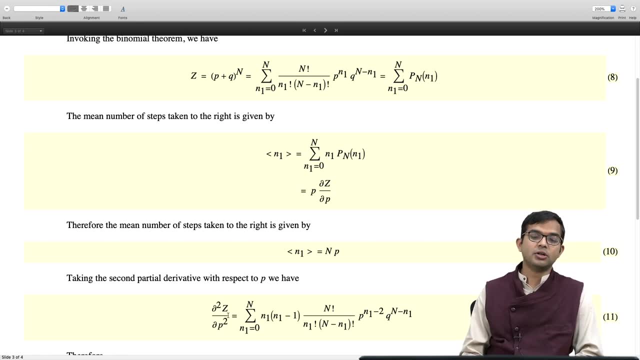 here is to find the average of N1 square. So here you just simply take a derivative of, with respect to p, once again of doh z by doh p. So in other words, you are looking at doh square, z by doh p square. the second derivative, partial derivative. and so now 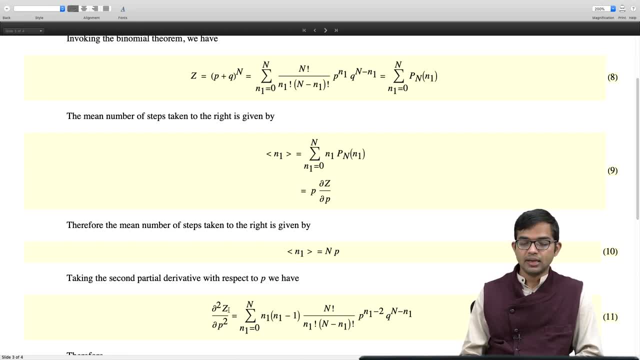 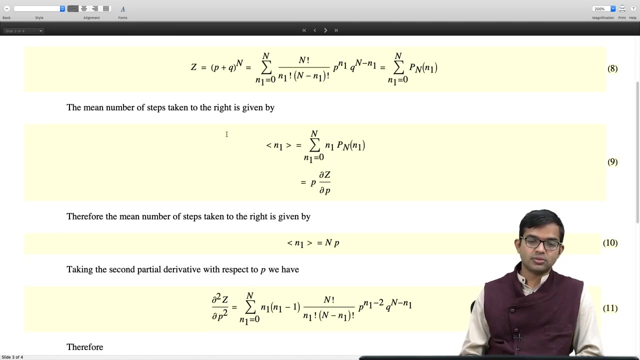 you see that you have N1 times N1 minus 1.. Right, So actually you are interested in N1 square. Ok Now, but we will see that using n1 information- and you know some trickery of this on the left hand side- we can actually evaluate this as well. So you should check this. what does? 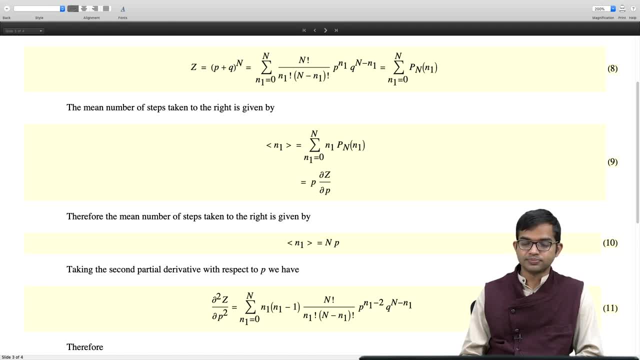 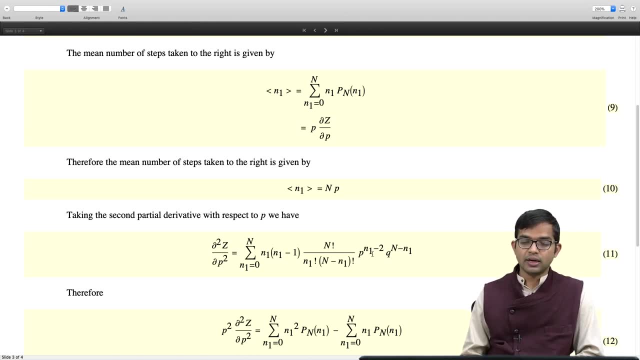 it involve Simply taking a derivative and over this sum and writing it explicitly like this: and then you multiply by p squared. now, When you multiply by p squared, you are going to get p to the n1. you have compensated appropriately for the loss in the power of p and then you 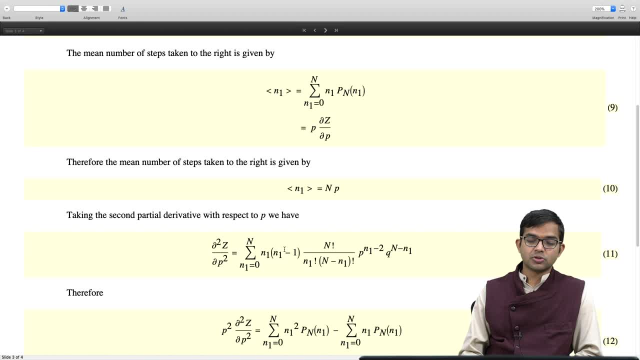 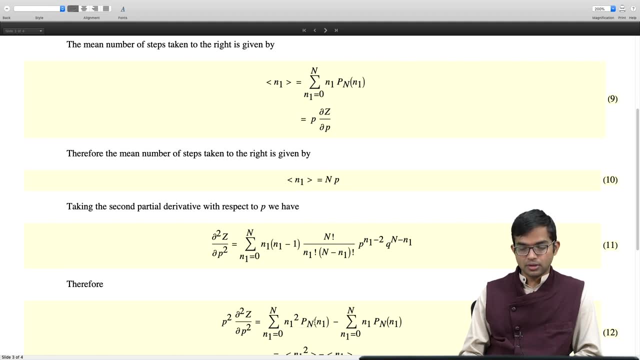 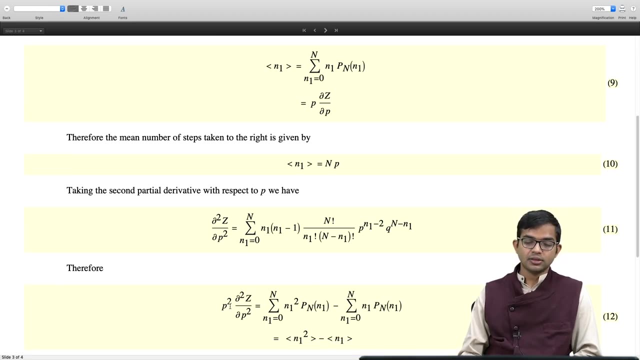 have to, you know, collect these terms. on the one hand you have n1 squared, but you have minus n1.. So you should verify this and check that indeed, you have n1 squared times the probability n of n1, minus n1 times pn of n1 and in fact this quantity p squared dou, squared z by dou. 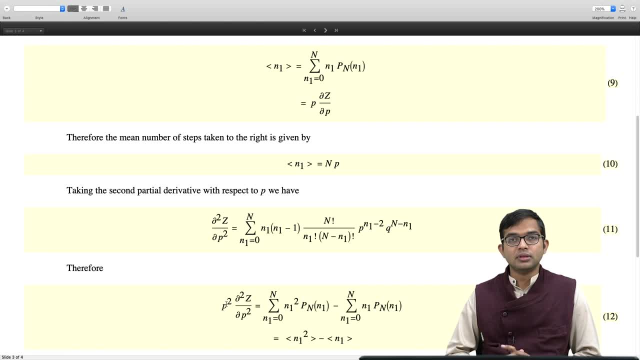 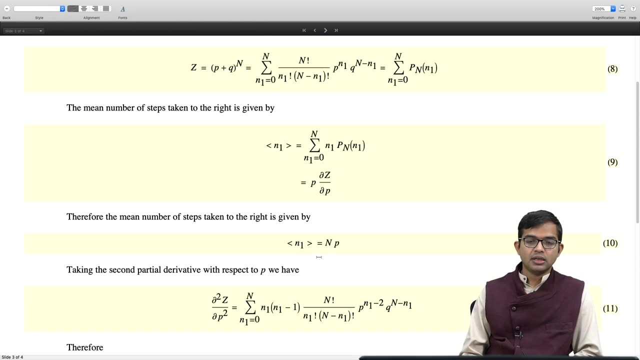 p squared is actually nothing but the variance of this random variable, n1.. n1 is the number of steps taken to the right. So this in turn yields, after putting p plus q, equal to 1. all you have to do is take this derivative n times p plus q, the whole to the n minus 1, and then again take another derivative. 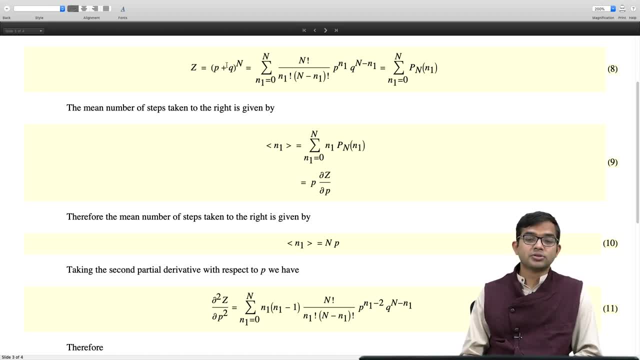 you will get n times n minus 1, times p plus q to the whole n minus 2, and then you put p plus q equal to 1.. You should reserve this stuff of putting p plus q equal to 1 to the last. This is some. 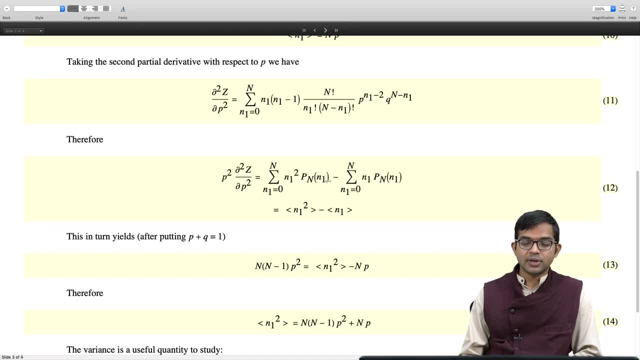 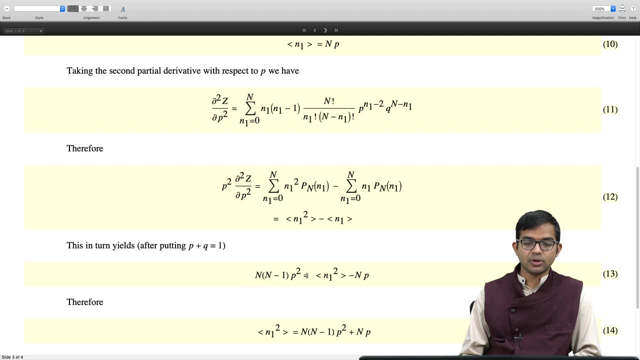 trickery Ponder over this And then you will see why it makes sense. Then you see, once you have this, you just plug in here n times n minus 1, p squared. So there is a second p also which comes in here, which comes in because you have p squared. 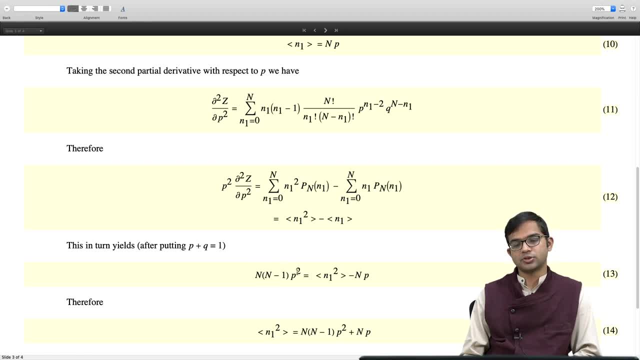 here, P squared sitting here, so you have n into n minus 1 times p squared is equal to average of n1 squared minus- which is unknown- minus n times p, because we already evaluated this And therefore You can see that average of n1 squared is actually now known. it is going to be just 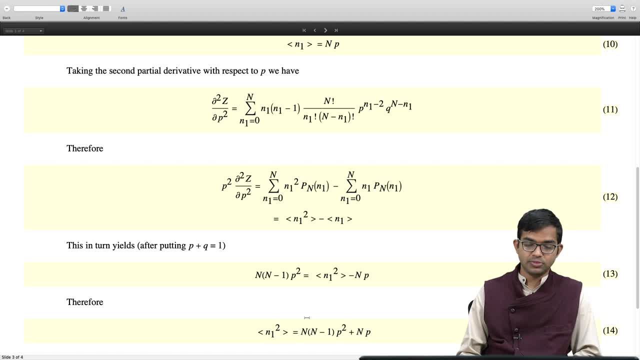 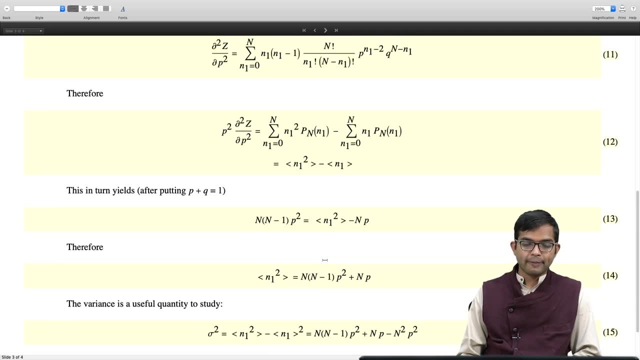 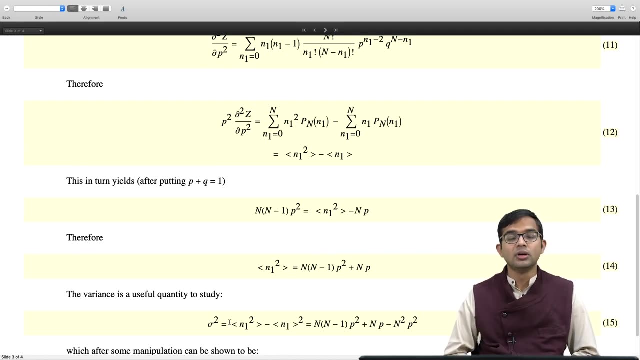 n into n minus 1 times p, squared plus n times p. So once we have this expression, we will go back and we will find out what is. we will find out what is. first of all, let us find the variance. sigma squared is equal to average. 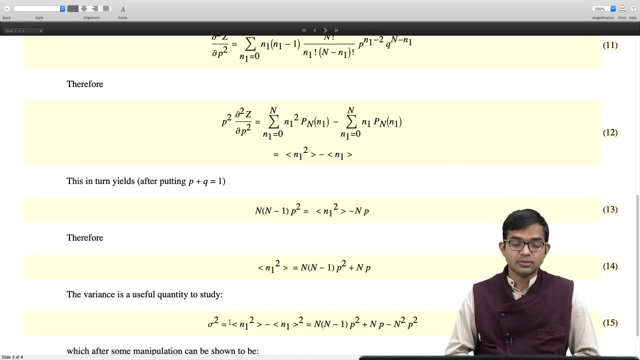 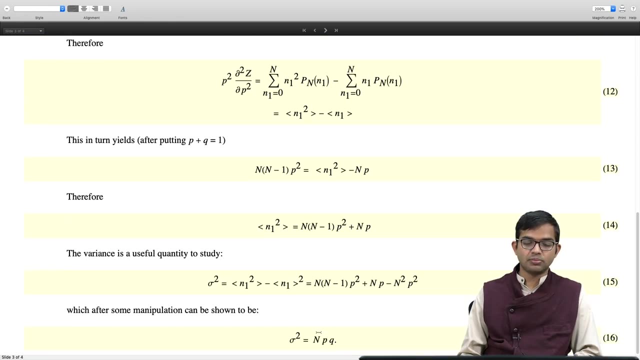 of n1 squared minus average of n1, the whole squared Right. So Check that this indeed makes sense. So, finally, the expression is just n times n minus 1 times p squared, plus n times p minus n squared p squared, which, after some manipulation, can be shown to be just simply n times p times. 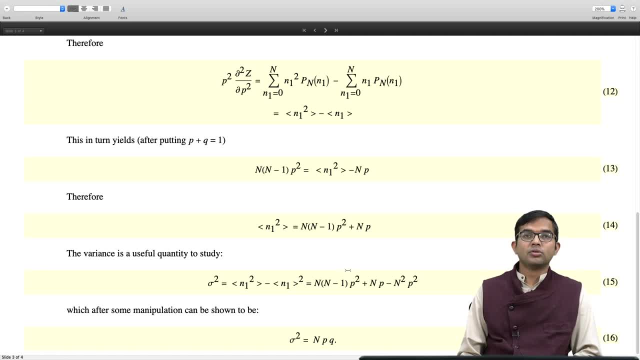 q. Okay, So this is for you to check this. all you have to do is use the fact that p plus q equal to 1 and then you can. you can show this. So this is homework. to go from equation 15 to equation 16 using p plus q. 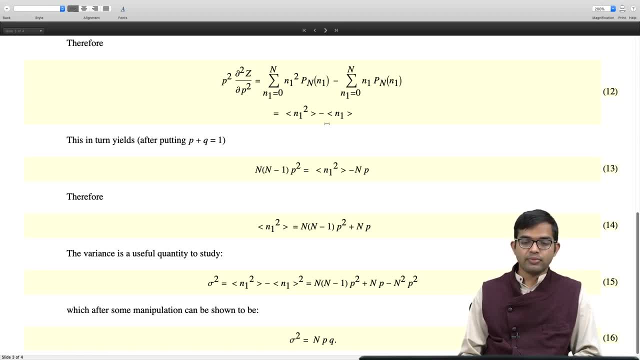 Okay, So we have obtained an expression for the mean of n1, we have obtained an expression for the mean of the square of n1.. Right, And therefore, using that, we have found the variance in n1.. Now, actually, we are interested in the mean and variance of the random variable m, which 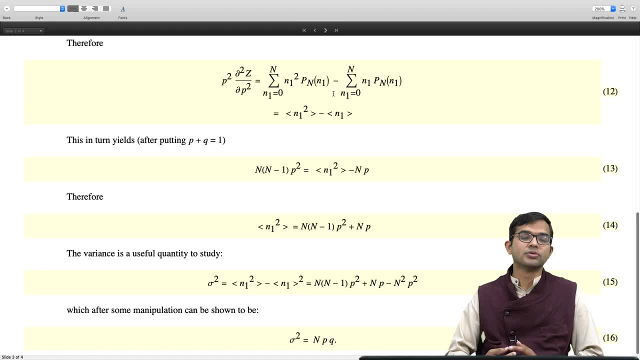 is, you know, the typical distance, which is a measure of the typical distance you are from the origin. So it is actually n minus n1 minus n2.. You can go ahead and compute this, you know, in terms of n2, and then you put in the variable. 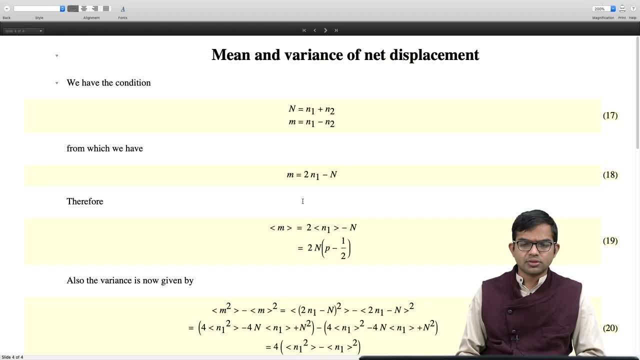 m as n1 minus n2, and that is one way of doing it. So another way is to do the following: right, you just solve for m in terms of n1.. So, since any, it is already given here, so now from which we have, m is equal to actually. 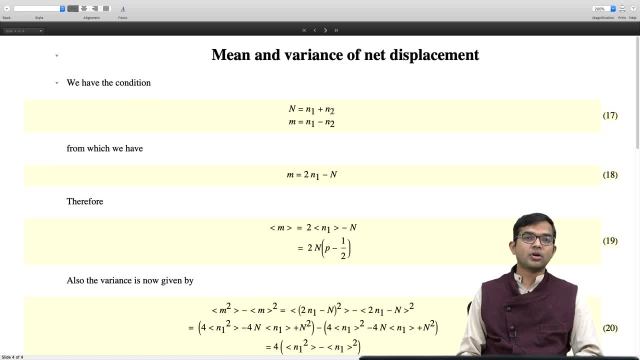 2. you eliminate n2 because n2. we have not really found out the information about its mean and variance, So you just compute. So this small m is equal to 2, n1 minus n. Now the average of m is simply 2 times the average of n1 minus capital N. 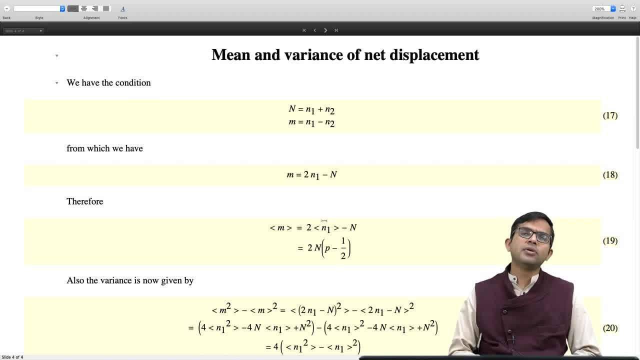 And the average of n1 we already found is n times p. By the way, the fact that the average of n1 is n times p is also very, very reasonable physically Right. So basically, what are you saying? You are saying that if you take one step to the right, the probability of going to the 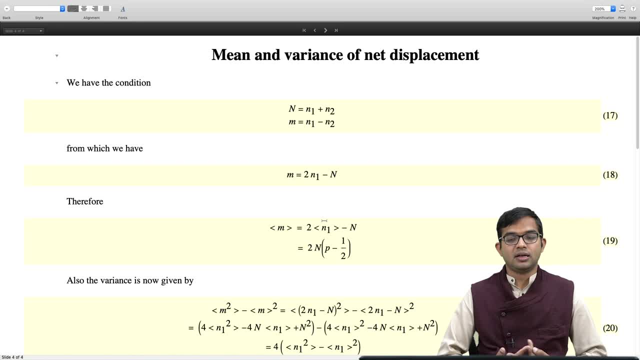 right is p. So the probability that after n1.. After capital N steps, the probability that you have taken, you know n, what is the number of, what is the average number of steps you have taken to the right, is just going to be capital N times p. 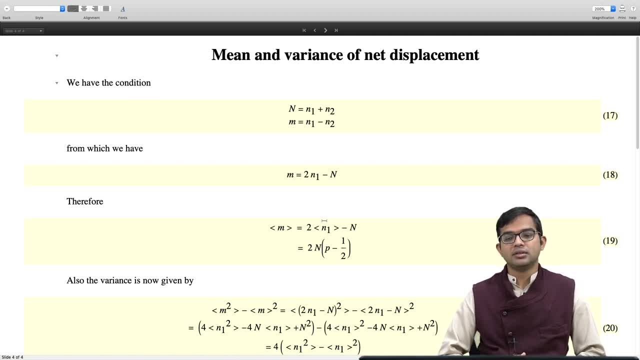 Right, Because in another way of thinking of that is, it is a bit like your. you know Monte Carlo in some sense, Right? So the average, you know the probability. if suppose you did not know what p is, how would you find out If you had a machine which would generate a random walk for you? you just simply count. 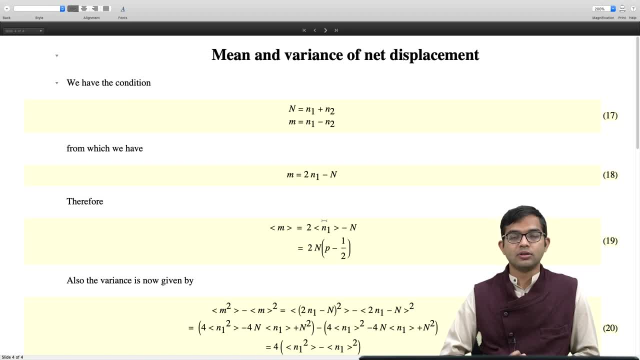 you after the first step, you know you will find out whether they went to the right or not. and then you get data for n steps and you ask yourself how many of these were to the right. So you will find a certain number, which actually is n1, and then so you will just divide n1. 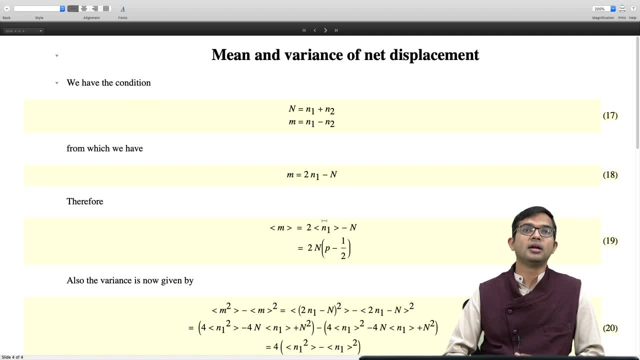 by capital N and say that should be the probability of going to the right Right. So that is, That is. That is in the spirit of a Monte Carlo like this is how we found out what is what is. you know like how many points fall inside a region. 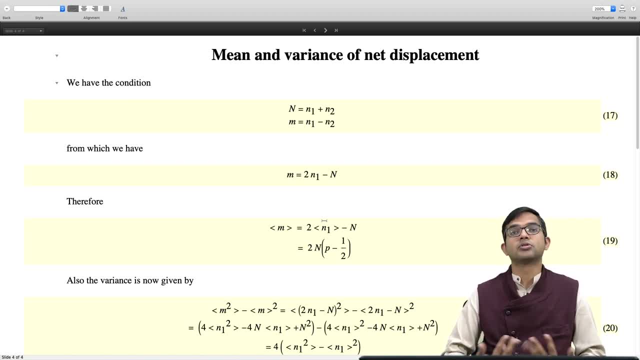 Right, If you want to compute the area of a certain region, for example, with respect to the total number of darts thrown, and so on. Right And so, in fact, if you want to find out whether how biased the coin is, this is would be the. 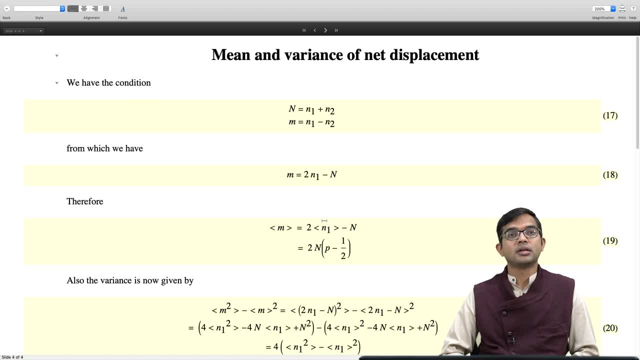 method Right, You just toss it and then you find that it has. do you get heads or tails Right? You get tails, then you find that again. then you keep on counting. So if you take a very large number of trials of this and you are finding that actually 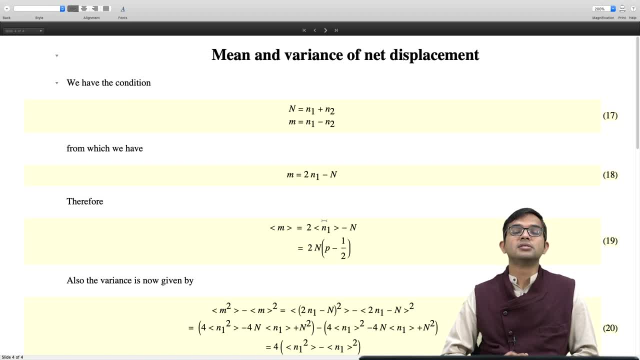 65 out of 100 are heads. So then you say that it is a biased coin. it is not a. it is not 0.5 and 0.5, but actually it is 0.61.. So that is going on here. 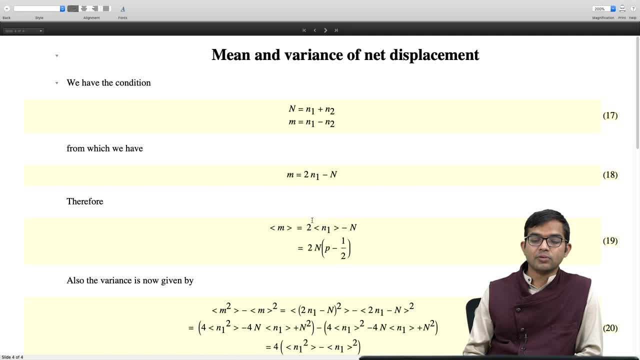 So now we have, once you have n1 average of n1, you can also quickly find the average of m. It is simply given by 2 times n, times p minus a half. So the variance is a little more involved, the computation of variance, but not necessarily. 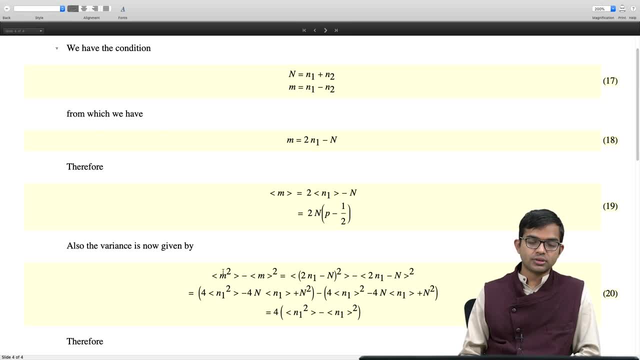 out of reach. All you have to do is expand this. So then you have 2n1 minus n- the whole square, minus 2n1 minus n- average of this, the whole square. Then you carefully pull out these factors, Right? So then you have 4 times. you know 4 can come out of the average. 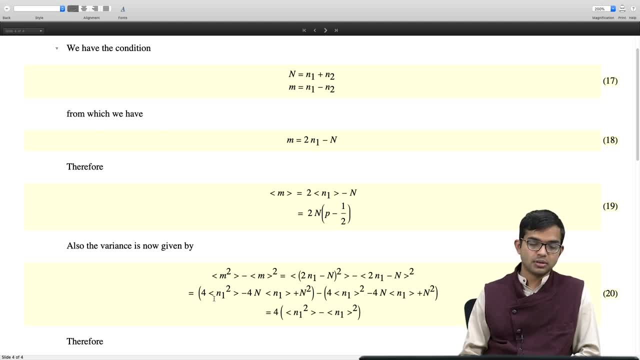 This is the average. This is the average Right, So it does not matter. So n1 square minus 4n times average of n1 plus n square minus 4 times n1. average the whole square minus 4n times n1. average plus n square. 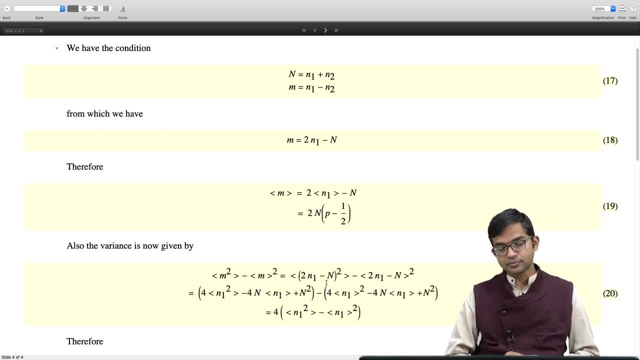 If you collect all these terms carefully, so you will find that in fact, the variance of m is related to the variance of n1 and it is just a matter of a factor of 4.. So just 4 times the variance in n1 is the variance of m. 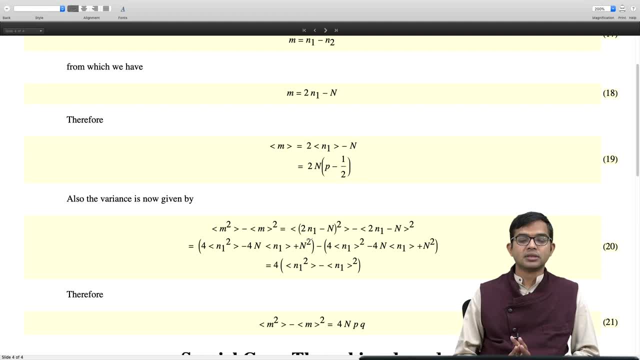 So you can immediately write down the answer, which is the variance in m is actually simply 4 times n times p times q, and its mean is 2 times n times p minus a half. So one immediate thing you would observe is, of course, what happens when p equal to half. 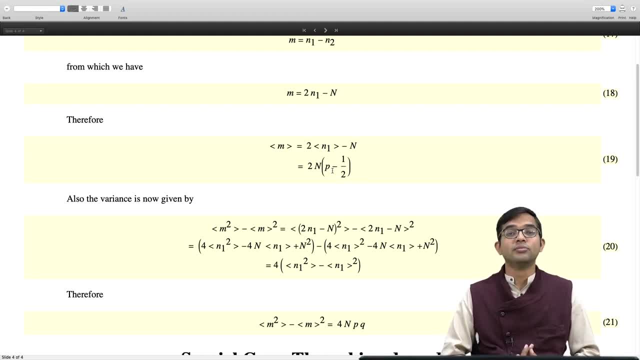 for the unbiased coin tosser or a random walker, So basically somebody who treats both directions, you know, equally carefully or equally carelessly. They do not care. They do not care where they are going. So with probability half if he is going to the right and with probability half he goes. 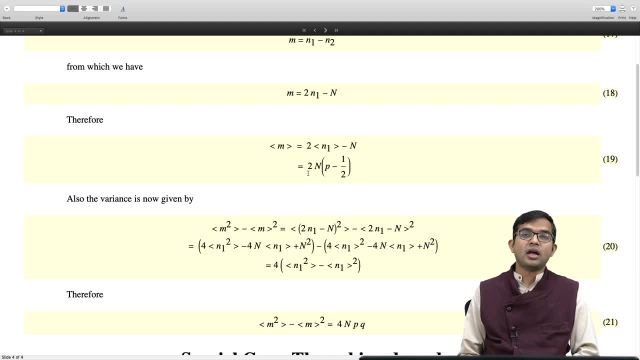 to the left, Then on average you expect that after capital N number of steps he has basically moved not at all. He will be very close to the origin. So the mean is indeed at the origin. There is no drift. And but the spread is, it turns out, is actually the more interesting quantity when you consider. 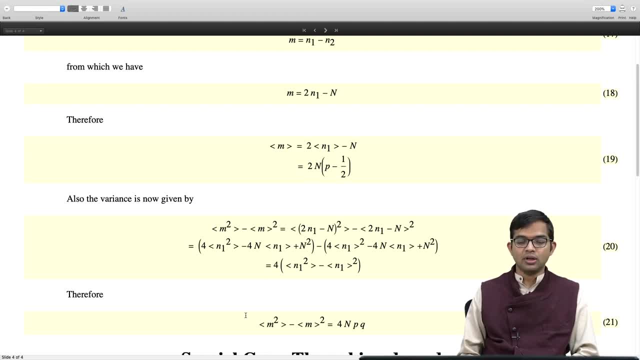 this: So, although the mean of this random variable is 0. There, But the variance will turn out to be n, So, in fact, so that is typically how far away he is going to be from the origin. He is not going to be sitting on the origin, like the mean seems to suggest. 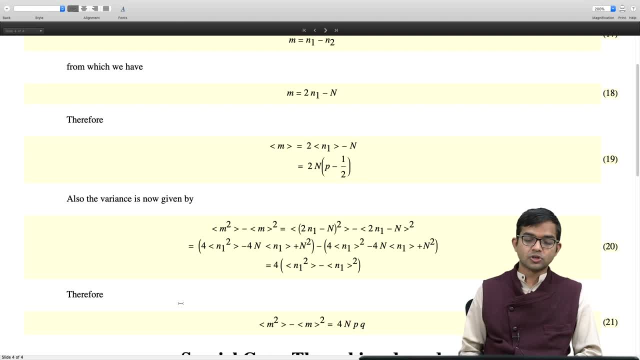 So, in fact, it is the variance that counts, So you have to take the square root of this, and so he is actually going to be very likely close to a distance of square root n away. It could on the right side or to the left. 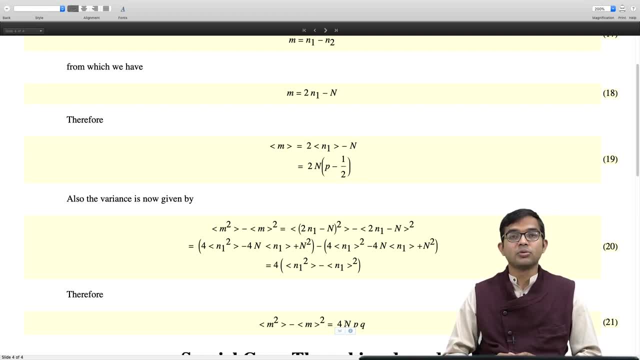 That cannot be ascertained. But but he is not going to be on the origin. So this is actually an example of how you know the mean of a distribution is not necessarily always the most meaningful quantity. Sometimes it is actually the variance, or the root of the variance, which is the standard deviation. 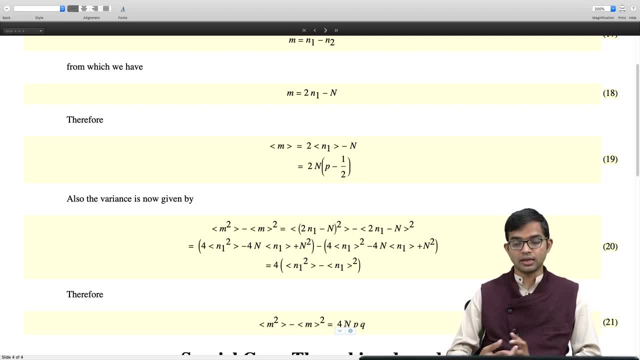 which carries more useful information than the mean, and so this is one such context where actually the typical distance of your random walker after n steps is actually square root n right. So let us look at this. this is a special case I have already talked about. 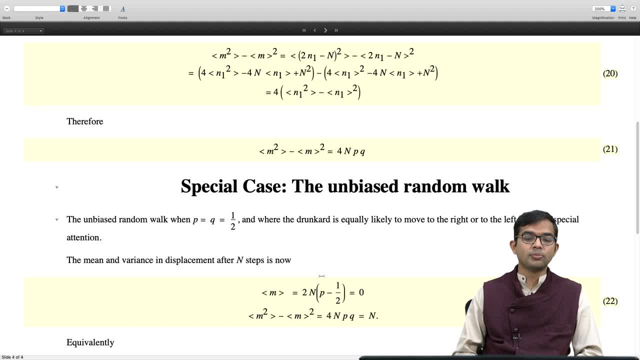 this, but let us do it more formally now. So if I put p equal to q, equal to half, so indeed average of m equal to 0, average of m square minus average of m, the whole square, average of m square, you know, with the bracket. 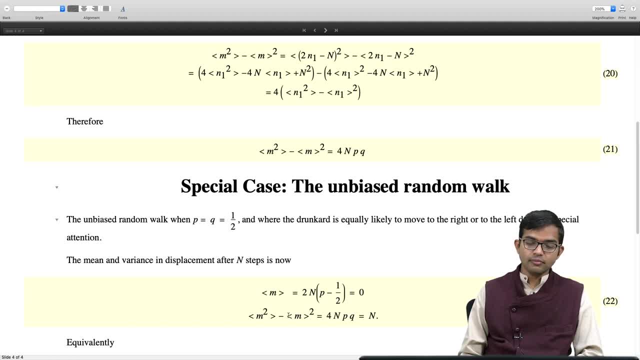 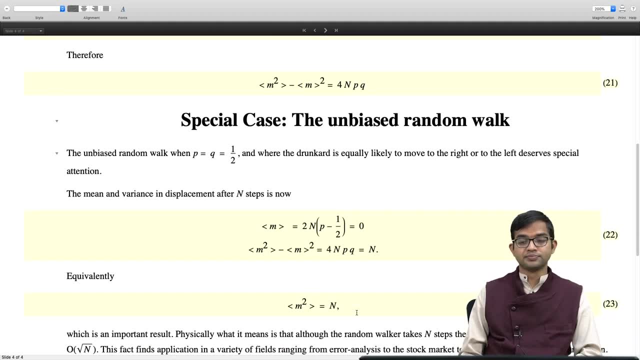 on square the. Okay, This angular brackets square, so this is equal to n and so, equivalently, this is a very, very important result. Ultimately, with all this simple set of arguments which seem very logical, we have managed to show very, very important result, which appears in all kinds of context. 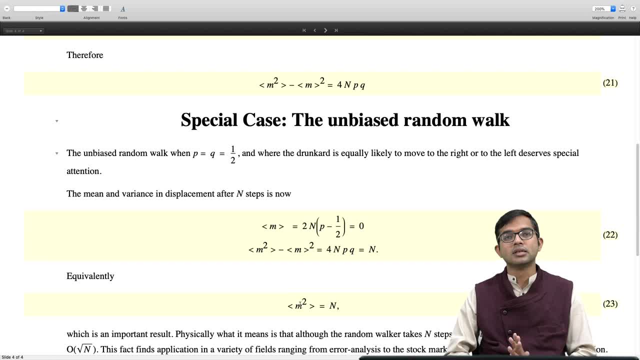 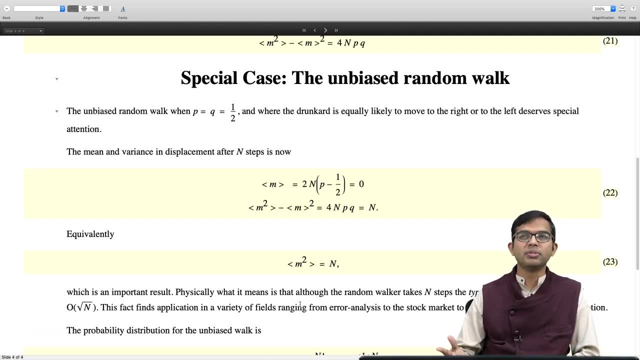 whenever there is a stochastic motion involved And that result is just: average of m square is equal to n. So if you take capital N steps, subtract basically, you are moving only square root of n. if you are a random walker, right? So if you have no purpose in life and if you are just simply exploring every direction, 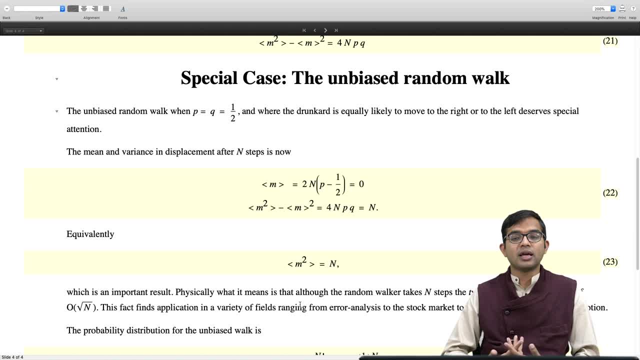 so you can imagine that. you know, although you take n steps, you would only go square root of n If on, and the best you can do is, of course, to go n right. so if it is of order n, it means that you are more or less going. you know all n steps. 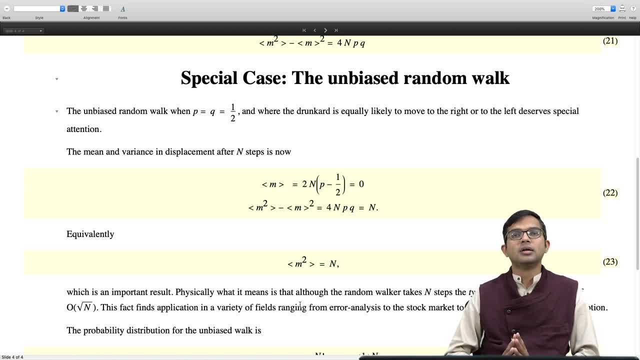 Okay, Okay, Okay. So all your steps, every step that you take, does count for your overall motion. So, and that is what is called a ballistic motion, and this is called a diffusive motion for a reason which we will show in a moment.